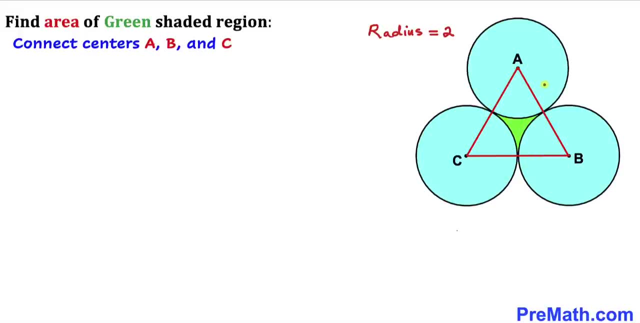 And now we know that the radius for all these circles is 2.. So this is 2.. This radius is 2.. This radius is 2.. Likewise, this is 2 across the board. Therefore, this total distance A- B is going to be 2 plus 2 is going to be 4.. Likewise, this distance. 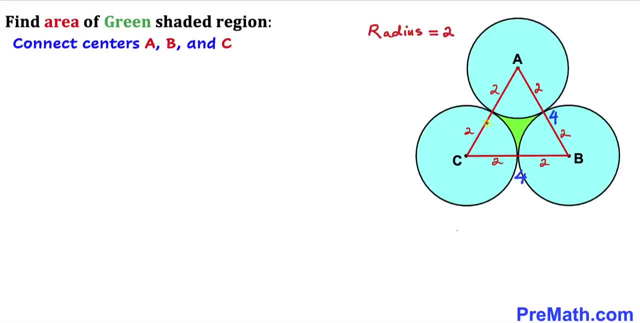 B, C is going to be 4 units And this distance, A- C, is going to be 4 units as'Well'. So therefore we can see there that our this triangle ABC is an equilateral triangle, Since all these side lengths of this triangle ABC is 4.. And we know that all the angles in an equilateral triangle are 60 degree each, This is 60 degree 15, and this has 60 degree and the triangle ABC is 60 degree. So the aim is to really be able to contain these triangles. eventually, If we have the triangle ABC and we have the angle ABC, it versus this triangle just greater then this triangle, there is a difference. 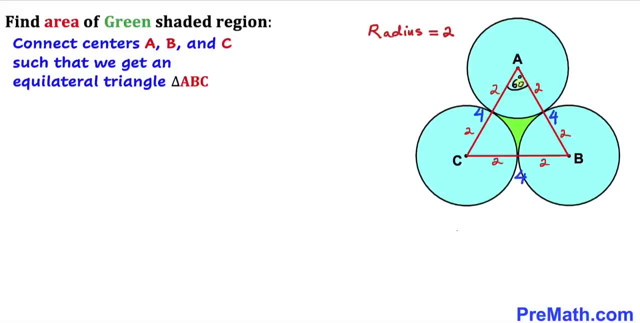 that unnatural mystery in each of these directions. Now let's see theánhangles here. For example, the angles here are 60 degree and the angles have 90 degree. this one is 60 degrees and likewise this is going to be 60 degrees each. and if we add all these, 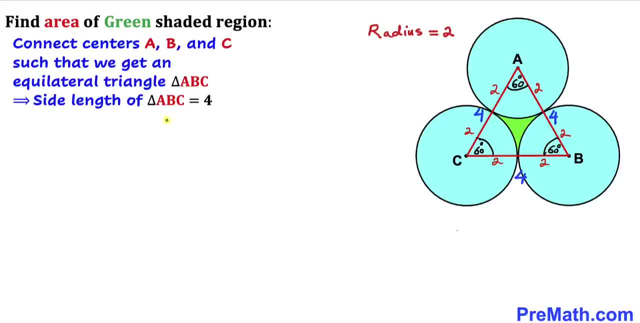 triangles, they must add up to 180 degrees and once again, just keep in your mind that the side length of this triangle ABC is four units. and here's our next step. let's focus on this equilateral triangle ABC. and here I have copied down this equilateral triangle ABC, and now we are going to. 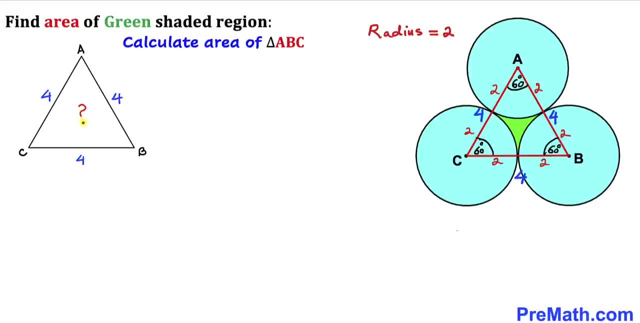 calculate the area of this triangle, ABC. and now let's recall the area of an equilateral triangle formula. in this case, area is going to be square root of three times a square divided by four, where this a represents the side length of this equilateral triangle. so therefore, a value is: 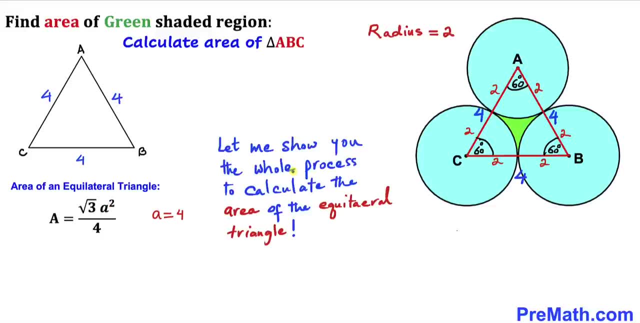 going to be the side length of this equilateral triangle. However, I have decided to show you the whole process to calculate the area of this equilateral triangle step by step. and now let's recall the area of a triangle. formula: area equals to a half time base times the height, and in our case, our base is four, if somehow we can figure. 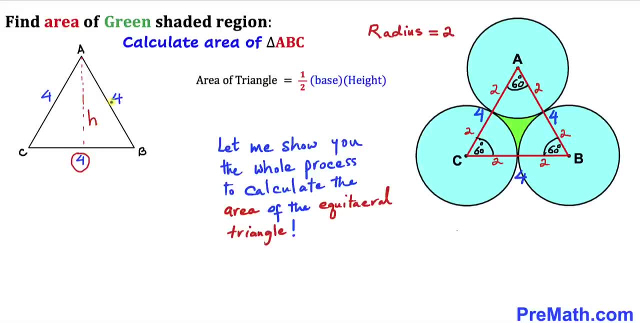 out this height h, we can easily find the area of this equilateral triangle a, b, c. so therefore I have dropped this perpendicular a d on this side b c. so therefore the side length c, d and b d are equal in length. we know the whole length is four, so therefore this side length is: 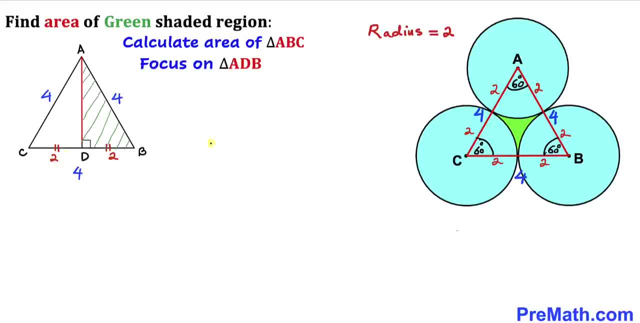 going to be two and this side length is going to be a two as well. and now let's focus on this triangle a, d, b and we are going to calculate this side h with this a d in this triangle and since this triangle a, d, b is a right triangle, so 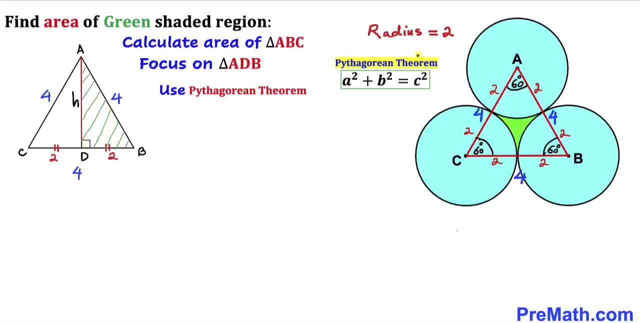 therefore, we are going to use the Pythagorean theorem, and here's our Pythagorean theorem: a square plus b square equal to c square, in our case, this longest leg, this a- b is I'm going to call side c. I'm going to call this side a and this side b. so let's go ahead and fill in the blanks. 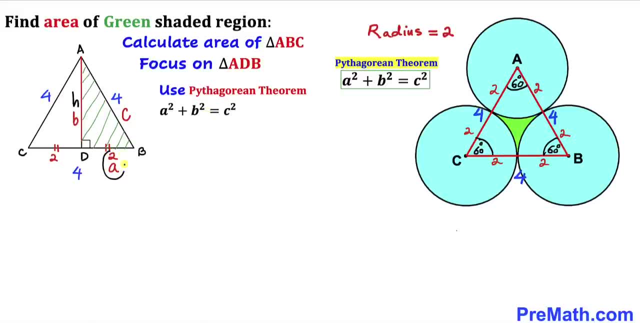 this Pythagorean formula: in our case, a is a, two, c is four and b is our h. so this is going to become two square plus this is going to become h. square equals to four square. if we simplify this thing, this turns out to be a four. 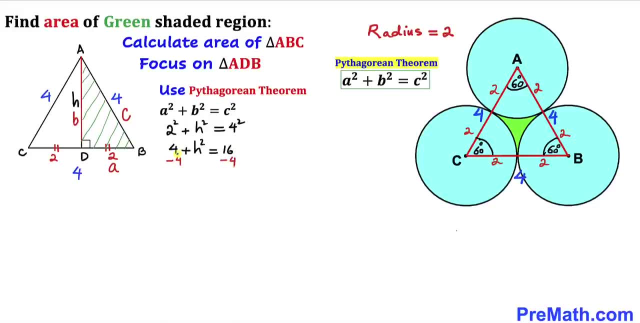 plus h square equals to sixteen. let's subtract four from both sides. this is gone, so our h square value turns out to be twelve. let's undo this square by taking the square root both sides. so therefore our h value is going to be equal to- and here I have. 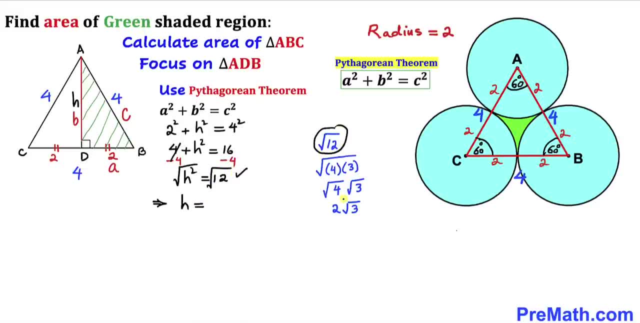 simplified this square root of twelve and it turns out to be two times a square root of three. so I'm going to write down over here: two times a square root of three. so therefore, our this height h turns out to be two times a square root of three. and now let's go ahead and calculate the area of this. 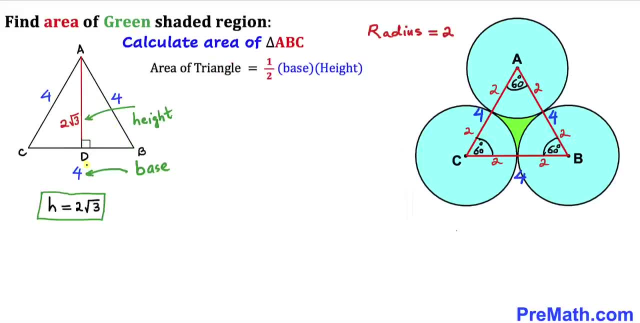 equilateral triangle ABC, and we know that this would be the distance between an. our base is 4 units and our height is 2 times square root of 3, and here's our area of a triangle formula. so let's go ahead and figure out that one so area is: 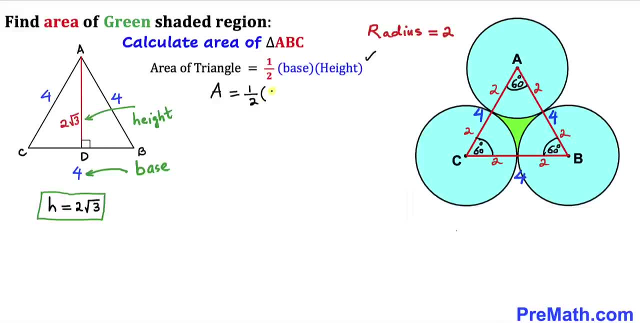 going to be a half times. the base in our case is 4 and our height is 2 times square root of 3 and if we simplify, this cancels out with this 2, so area of this equilateral triangle turns out to be 4 times the square root of 3. so 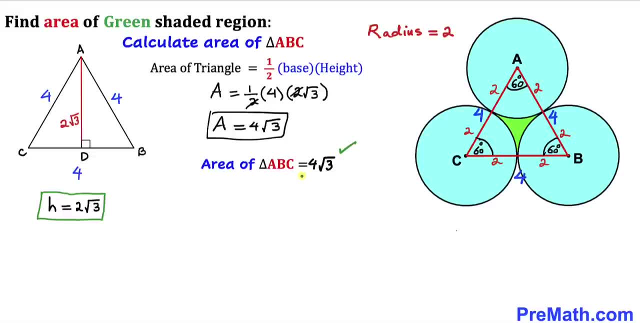 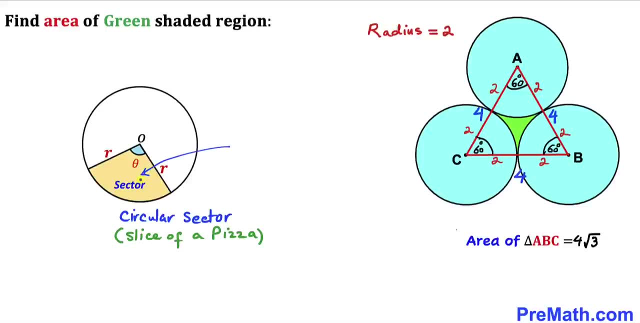 therefore, the area of this equilateral triangle ABC turns out to be 4 times the square root of 3.. now let's focus on this circular slice of this circle, and this slice is called the circular sector, and in our case, this is one of our this. 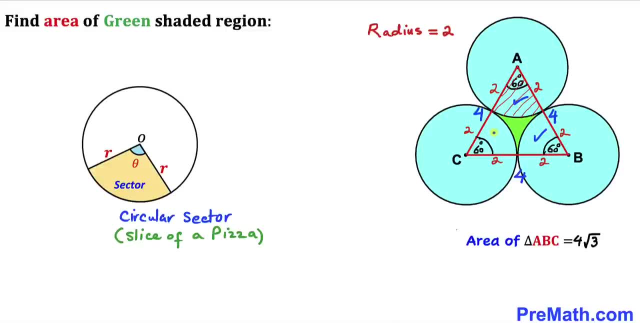 sectors, and this is the second one, and this is the third one. and now let's make an observation. we can see that this, our green shaded region in between these circles, is equal to the area of this bigger equilateral triangle, minus three times the area of these sectors, since we have a three of these sectors and just 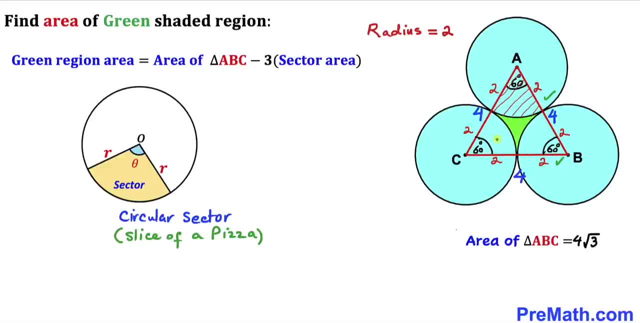 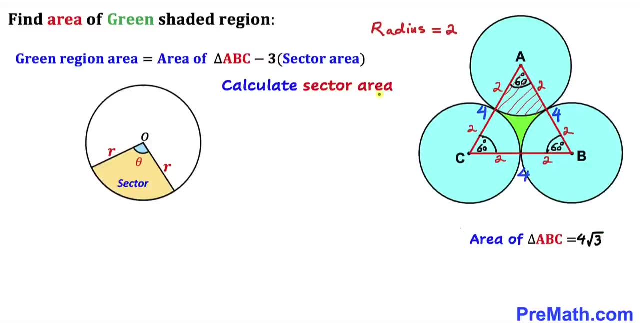 keep in your mind that all these three sectors are identical. and since we already figured out the area of this triangle ABC, so therefore let's go ahead and calculate the sector area. and now let's recall the sector area formula. sector area equals to theta divided by 360 degrees times a pi R square, where 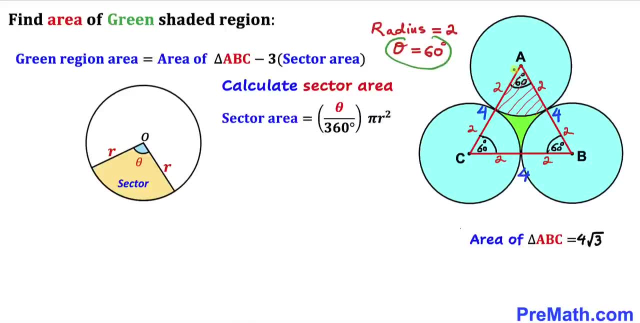 our angle theta is 60 degrees, as you can see over here, and our radius is equal to theta divided by 360 degrees times pi. R square, where our angle theta is 60 degrees, as you can see over here, and our radius R is 2. let's go ahead and fill in the blanks in this sector area formula. so: 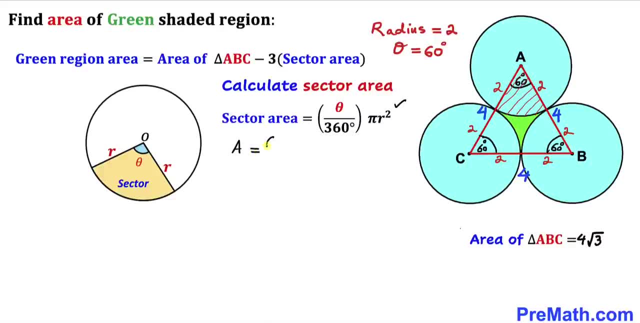 sector. area A is going to be theta in our case is 60 degrees divided by 360 degrees times pi and R, in our case is 2, so this is going to become 2 square. now we can see 60 degrees divided by 360 degrees is going to reduce to 1 divided.